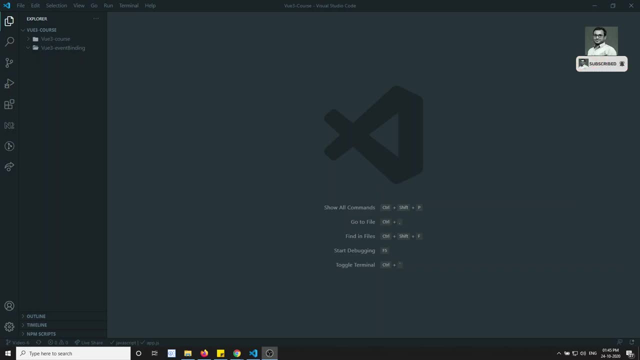 Hi friends, this is Leela. Welcome to my channel. In the previous video we have seen the V-HTML directive. we have seen and also we have seen how to write the methods in the Vuejs Vue 3 course we have seen. right Now in this video we will see about the event binding, So how we can apply. 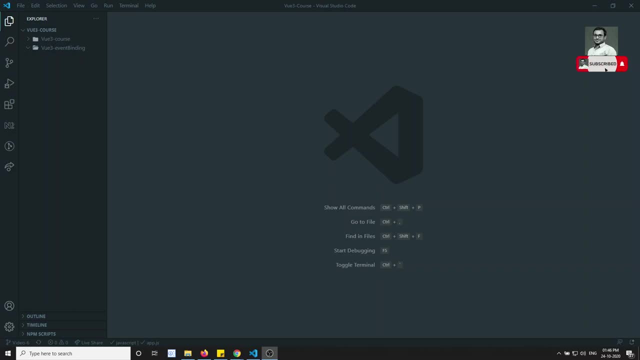 the event binding in the Vuejs. So in Angular we have seen how to apply the event binding, So we have used the brackets of click, like that right. So in the same scenario, how we can use the, I hope we can use the event binding in the Vuejs, Let's see in this video. So before 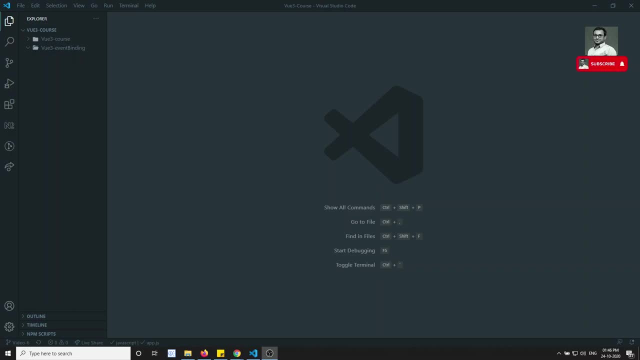 continuing to this video. if you are coming first time to channel here, please do support me by subscribing to my channel so that I will be posting more and more front-end development courses. Okay, now I took a new folder. Okay, instead of this one, so these are previous things I took. 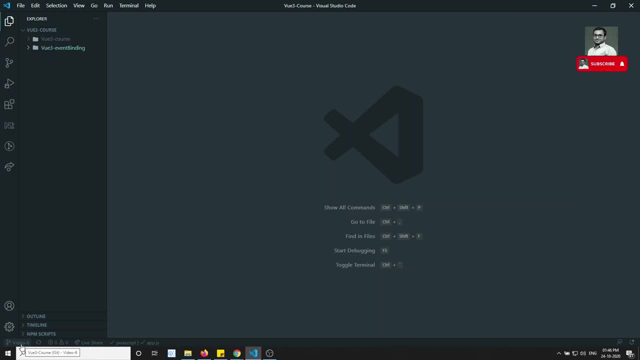 a new folder and I am creating. I have created a new branch with the name video-6 so that for every video you will be having a new. we will be having a branch with that video number name so that you can go to the particular branch and you can see the code for. 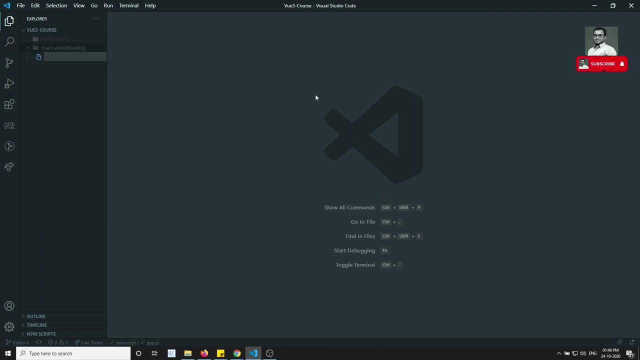 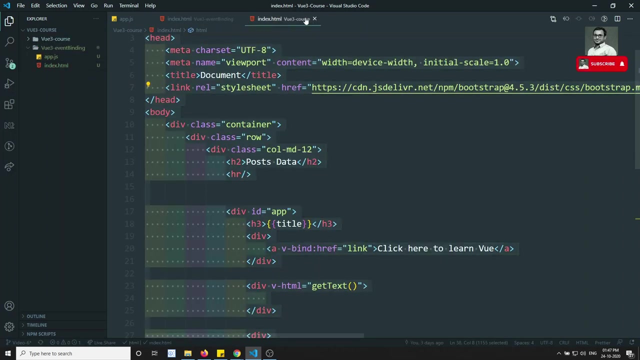 there. Okay, now in this one, let's try to create a file. So same thing, like that: appjs and indexhtml. the same scenario will create that data. okay, now, indexhtml. I can go to the previous indexhtml. what I have written and I will. I will write the. I will paste the same code and now I will remove. 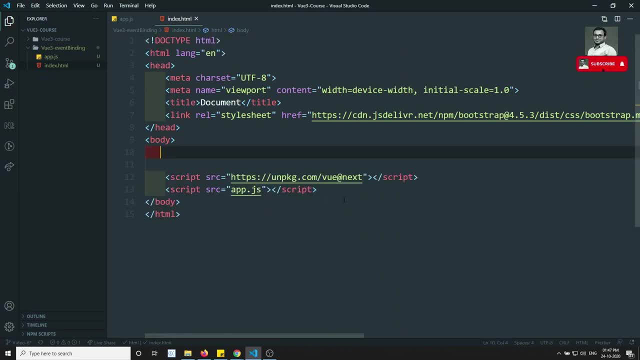 these all the code. Okay, the basic html. so this is the basic html boilerplate template. now we have included the vjs3 and appjs is included here. here the bootstrap is there. this is this is the simple thing. what i will try to do here. i will try to create a container and i will try to have call mod 12. 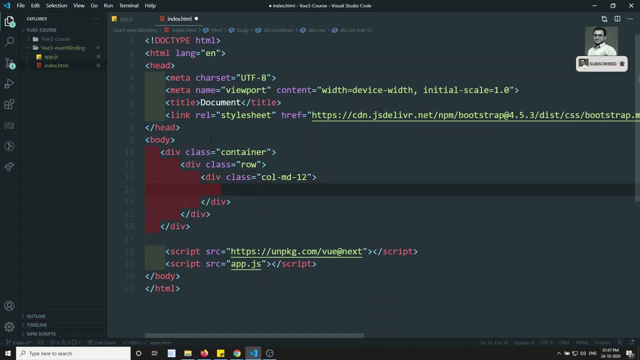 so i will be having this container and this call mod 12, and now what i will try to do is i will try to create two buttons, so i will take class is equal to mtf and three, just i am applying some margin top and i will create here two buttons. so what i will try to do is i will create one button. 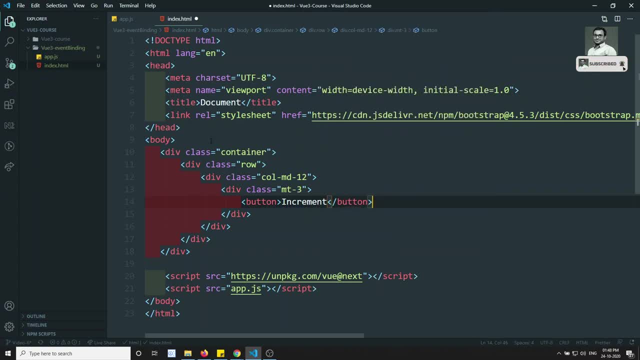 with increment button and i will give some gap. we can give some gap using an ampersand, nbsp, so it will give one one word, one one letter gap. and now here, what i will try to do is increment. what i will do is i will create a button and i will create a button and i will create a button. 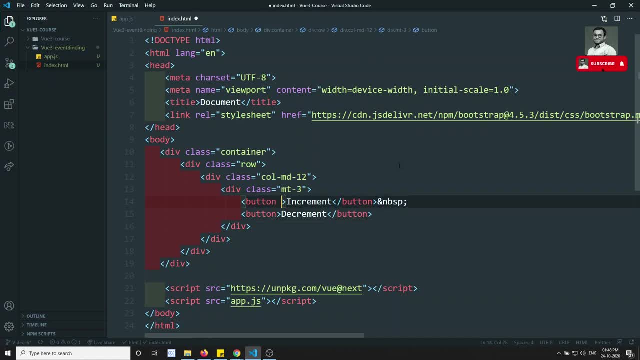 okay, so these are the two buttons which i am having: increment and decrement. so i will. i will try to do some cleaning, okay, so this one will be created. okay, so i have, i have created, uh, but two buttons. so i have just uh, added the css class button button i can, primarily so that the buttons look somewhat neat. 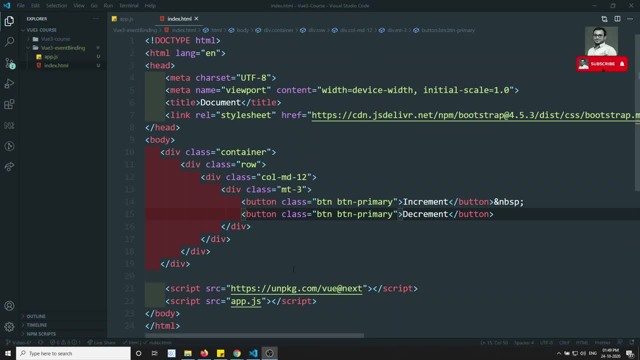 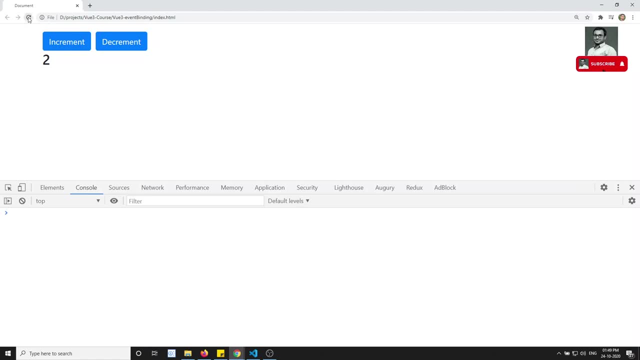 now we have added the buttons. right, let's see the output. let's see the output here, if i go and if i check the output here. so this is the output if i refresh it here. okay, yeah, so this is that: increment and decrement. we have got the two buttons. 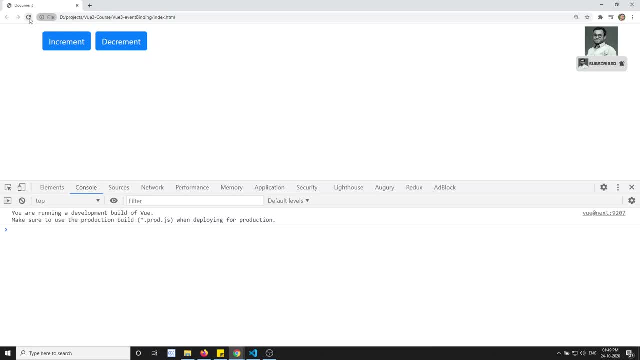 incremented decrement and what i will try to do is what i will try to do is: i will try to, i will, i will try to, i will try to add the event binding to this one. so on, upon clicking on this one, so i will increment one value and upon clicking on this button, i will decrement the value, so we. 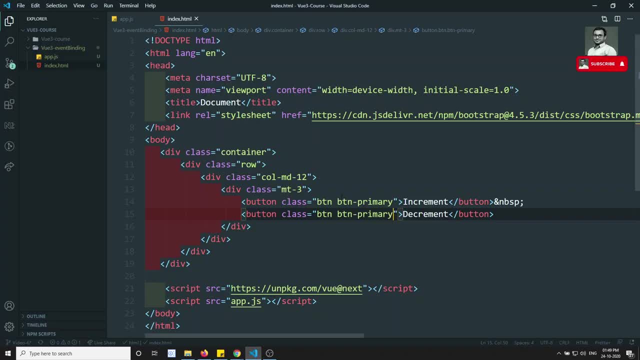 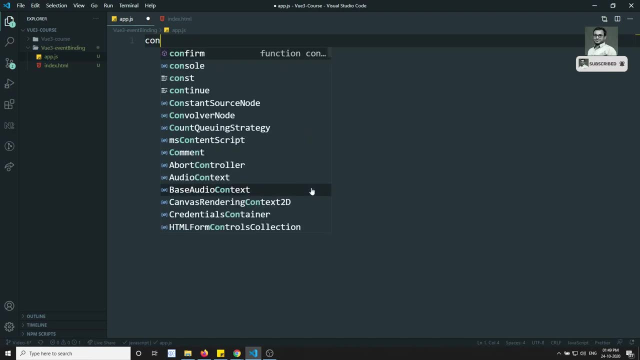 will try to implement the event binding. how we can implement the event binding is: let's go to the appjs. let's create constant. sorry, constant app is equal to view dot. these are things we have already discussed. how to create the app. you dot create app, so we let's write, let's write afterwards and app dot mount and we need to use 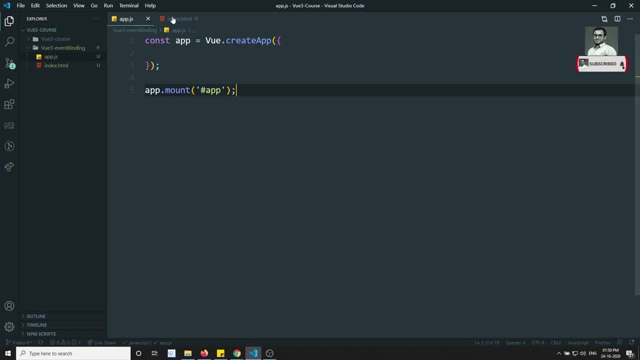 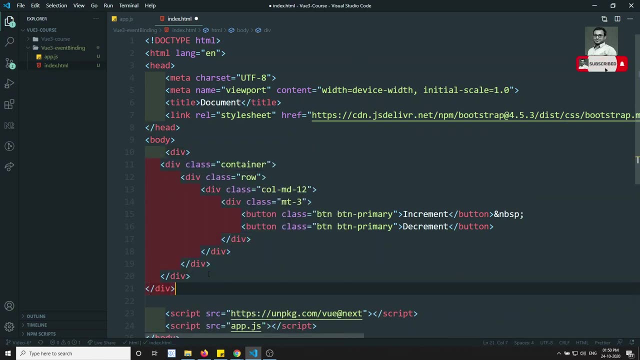 the identifier. okay, so up to where the vue js has to apply. so let's create one. do here, and i have created one. do here: let's try to give id. id is equal to app. okay, i have given id is equal to app. let's try to use like this: okay. 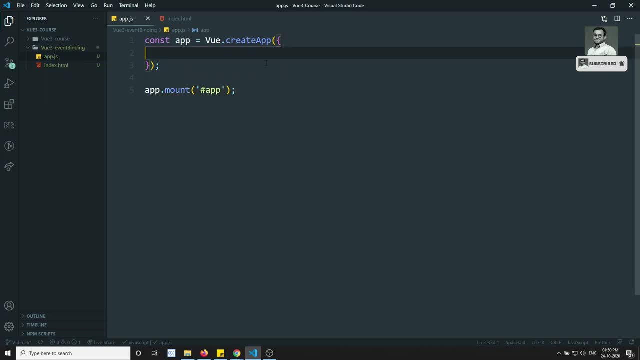 so this one is the. i have created a vjs instance and here let's try to have one data variable and here i can write return, and let's try to create one variable which is count 0. okay, it's an object. we are having one property with the count 0 and now i can. 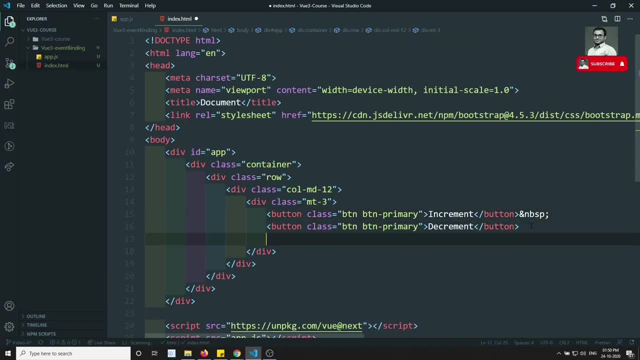 use this one directly in here, so what i can do is do count, so i will be showing the count. so, instead of being, i will use h2 or something like this, so that it will be little bit of bigger. now, if i refresh this one, what you'll be able to see is that you can see that i have a property called vizu. 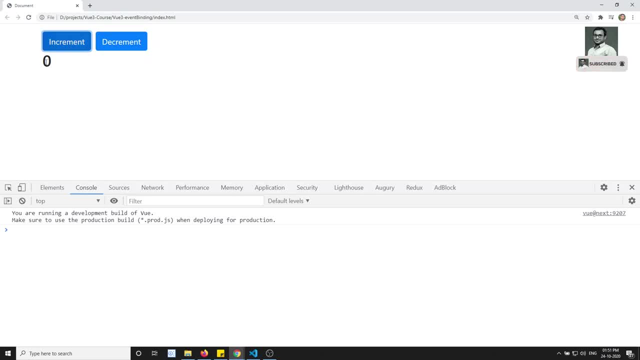 to see. you will be able to see zero the output. now, when i click on this button, this should increment to zero, to one, two, like this: when, upon clicking on this, it has to increment plus one and upon clicking on this decrement button, this count has to decrease minus one. okay, by. 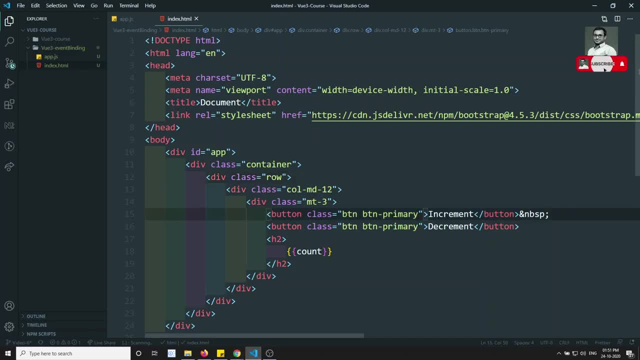 one and by one it has to increment. so how we can do now we need to apply the event. click for this one. so how we can apply the event: click for this one. so for applying this event, click how we can apply is how we can apply. is so in the view js, if you want to apply this one, how we can. 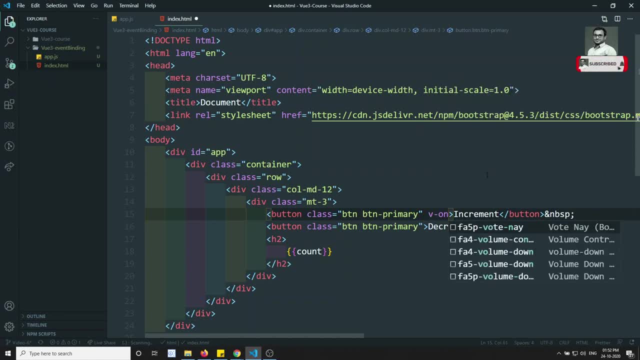 apply is v hyphen on directive. we need to use v hyphen on directive and we need to use click. okay, v hyphen on directive. on click, you can write the method. whatever the method you want to execute, you can write your own method. so i am writing on increment in the 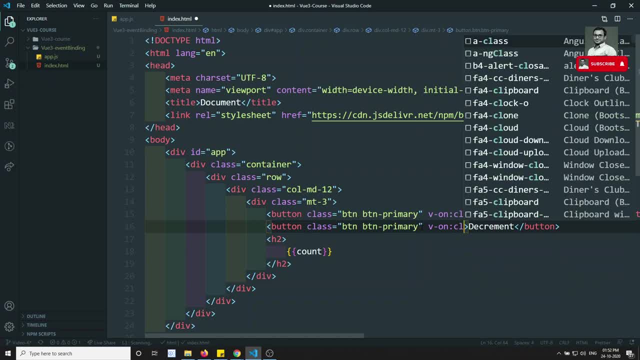 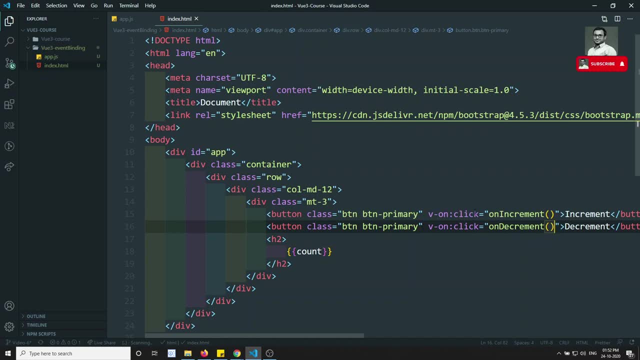 same scenario here. v hyphen on directive on click is equal to on decrement. okay, i have used another method for this one. so this click thing is nothing. but what we can say is: these are all the normal vanilla javascript event listeners only. so click change, we can write. 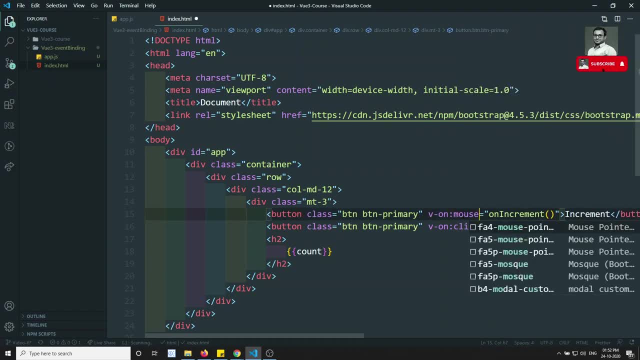 change mouse enter. these are all how we are using in the vanilla javascript. in the same scenario, the names will be the same. only so there is no need to. uh, there is, there is. there is no separate event binding names for this one. okay, so click a mouse enter, mouse leave, change key up key. press key enter. these are common, however, you. 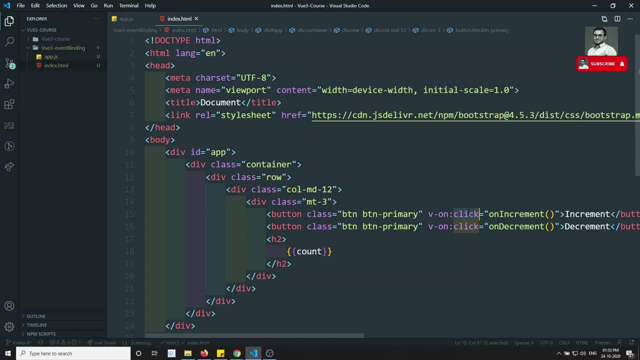 are using the vanilla javascript, the names. so same thing, we can use it here. so we have used v hyphen on directive on click, like this. we have used it right. so now we need to implement these two methods on increment, on decrement, how we can implement here, let's go. and if 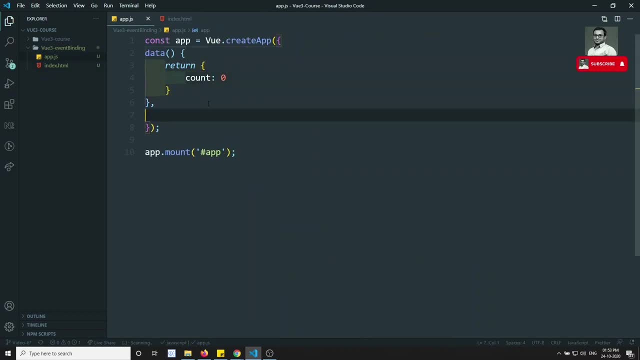 we need to implement the methods. what we need to do here: i need to write the method. so let's go here according to the methods. it's an object, okay, methods. what i need to write here on increment: so we have a method on increment and another method is nothing but so, comma, we need to. 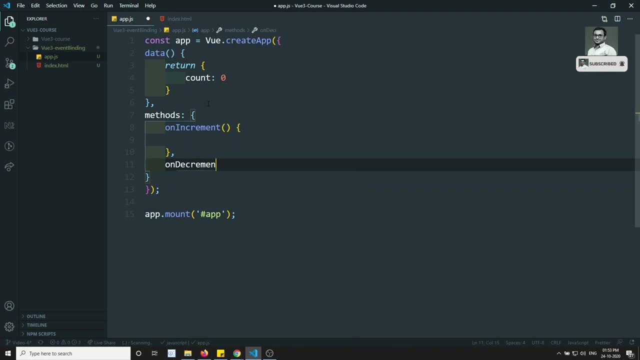 keep on decrement. okay, so this is another, another function. now what i need to do? so i need to increment this count by 1 on increment when, when the user clicks on the increment. so that means how we can access. we can access the count using this dot楣 lleg parts to content this dot. 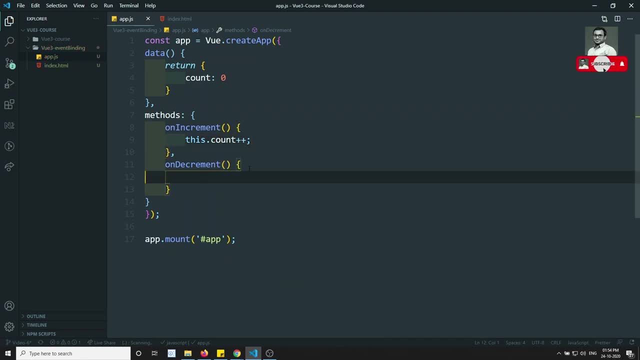 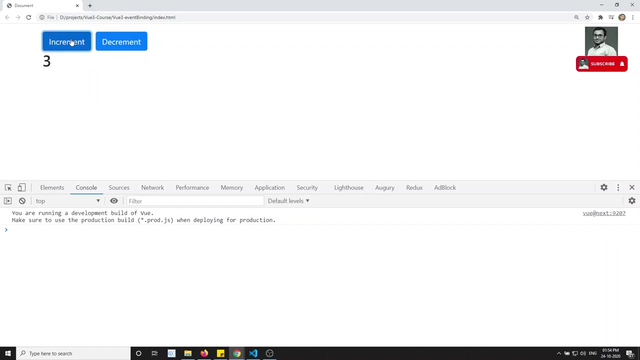 dot count plus plus. i have used this dot count plus plus and here how i can upgrade, is this: dot count minus, minus. okay, so i have incremented and i have decremented here. let's go and see the output. so if you click here and if i click on increment, you will be able to see that. 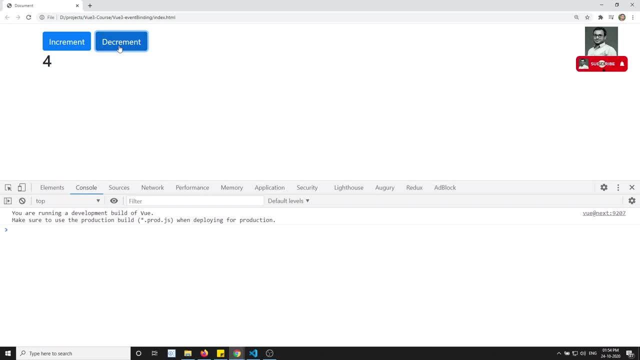 value is incrementing and if i click on decrement, you will be able to see that it is going on decrementing. if i click after zero, also, it go on to minus one minus two minus it like this. so if increment here, it will go on like this. okay, so so here, this is how we will be implementing the. 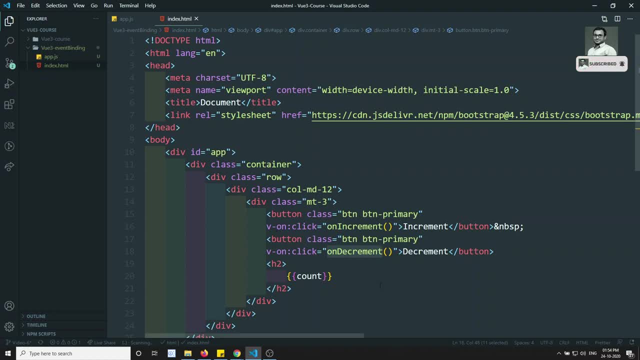 click events or whatever the events you want in the html elements using the in the vjs. so we need to implement it like this: we use the, we need to use the v-on directive on click and implement whatever the method you want or otherwise, what i can use if you, instead of calling this method, 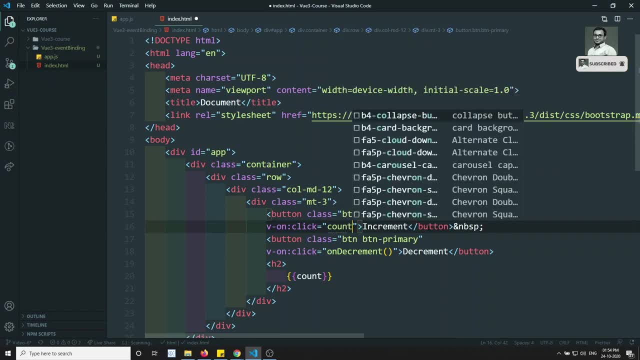 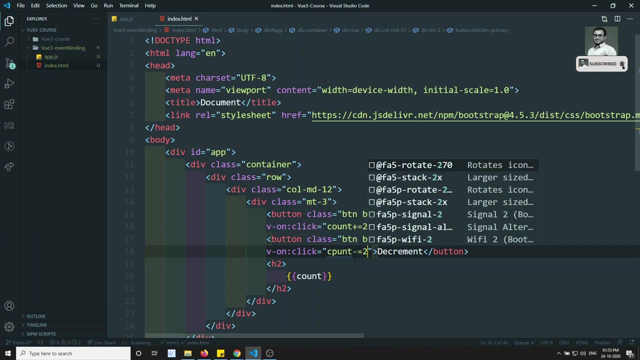 we can also write directly the code also here, so we can write count plus plus here and also you can write count minus minus also. count minus minus also. we can write. and also: if you uh, for example for checking also count plus is equal to two, that means, it will increment by two times. count minus is equal to two means it. 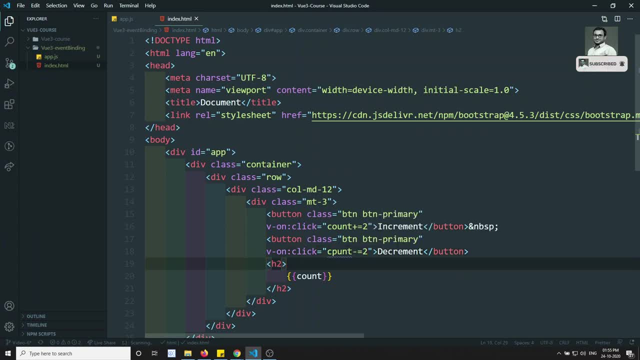 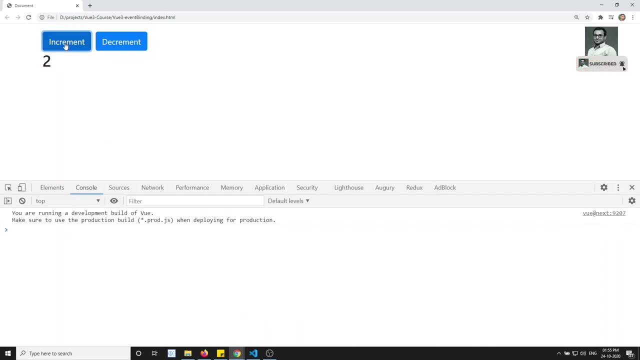 will increment by two times. so here, if i want to check, okay, if i want to check this one, so if i refresh this code and if i click here, see, you will be able to see that it is incrementing by two times. if i click here, it is decrementing by two times, okay. so this is how also we can write.